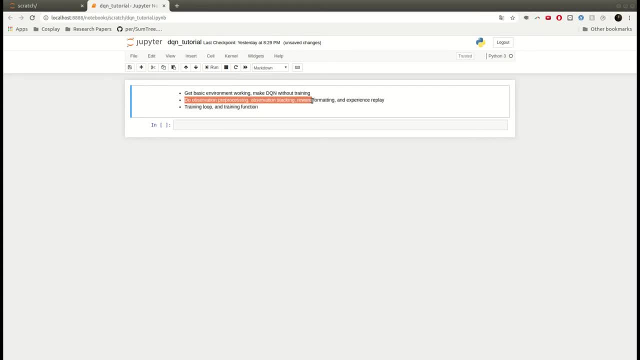 next video. after this you can expect to start working on some of the pre-processing for the data, the reward formatting and the experience replay- all the data, heavy stuff And then the video. after this one or after the next one, we'll start working on the actual training. 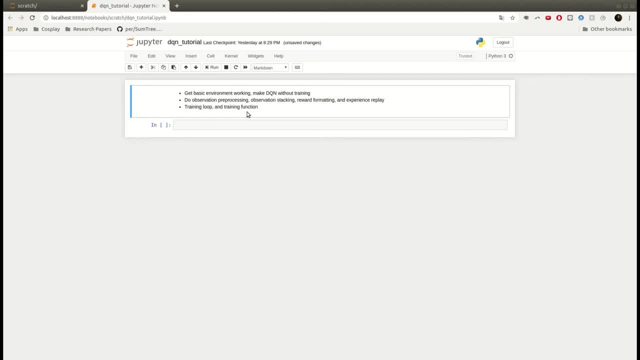 and go into how we actually train our model to do better. So, again, there's a lot to go over, so I want to dive right into it. The first thing are imports. We will be using PyTorch, You know. if you use TensorFlow, though, or something else, you should still be able to follow along. just 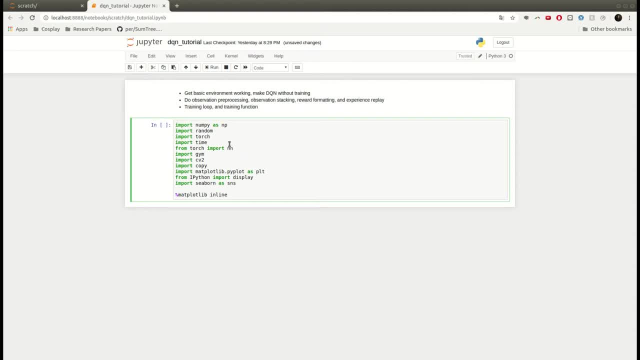 fine, The logic's all the same and I think hopefully the code should be fairly easy to understand and easy to translate to any other machine learning library, So no need to worry there. I think GIM first of all is OpenAI, is basically a way to use reinforcement learning. 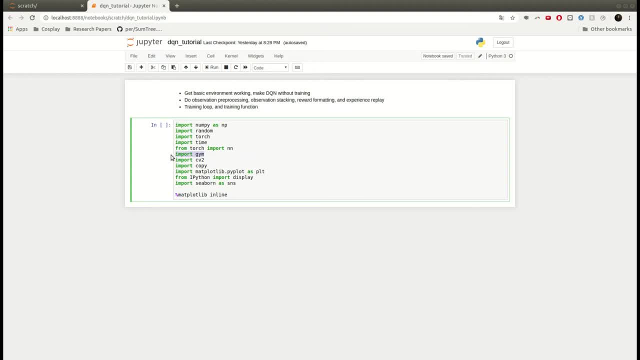 environments. GIM is basically a way to use reinforcement learning environments. It's basically a super easy way to use things like Atari environments or what not, so we don't have to set them up ourselves. CV2: we will be using for image pre-processing. 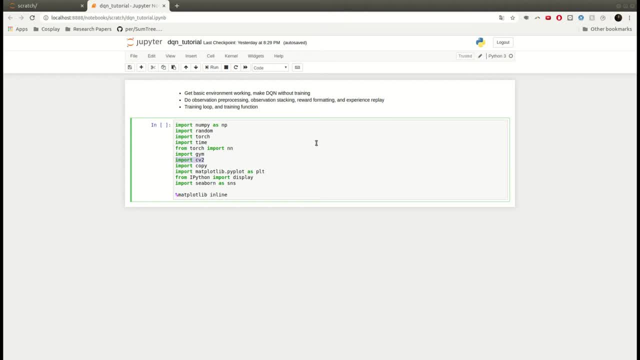 As we are playing Atari games, we get a 2D image. we need to be able to process that, And then matplotlib and Seaborn for plotting out any data we might want to look at after our run-throughs. Cool, so let's dive into it. Import that and the next thing we want to do. 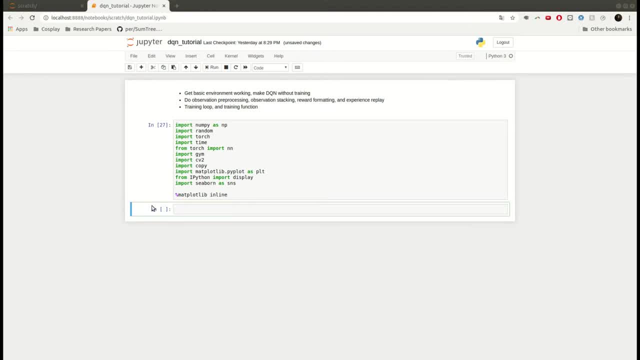 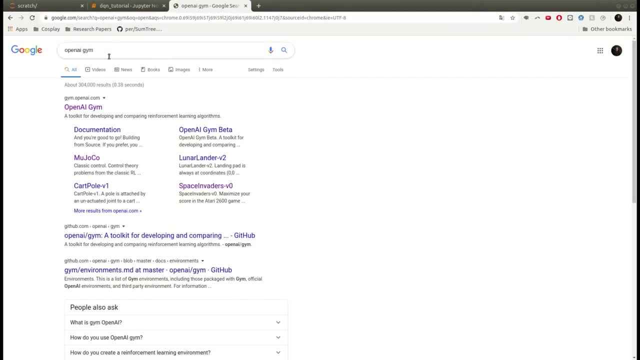 is make our first environment, which is actually super easy. All we have to do do is this: right, we say gymmake, and then we give the name of the environment we want. we can actually get a list of environments. we get type in openai, gym, gymopenaicom, and go to over to environments. 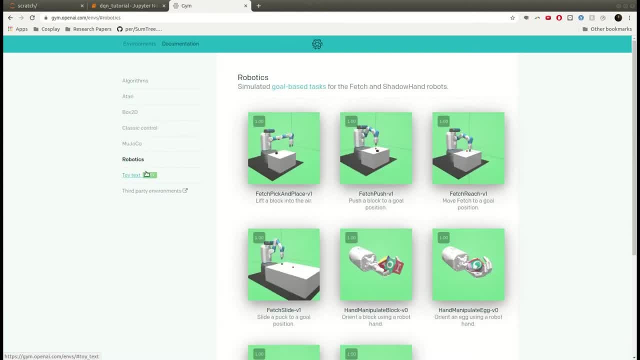 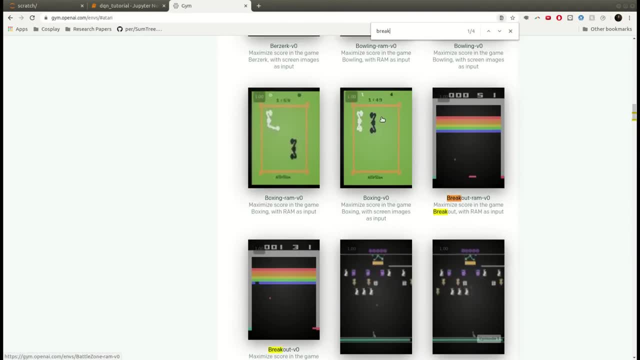 you can see there's lots of stuff here. we will be particularly interested in the atari games here we'll be starting out with breakout. if you've never seen breakout, it's a fairly simple game, essentially. it's right here. right, you're just trying to use your paddle to break the blocks. 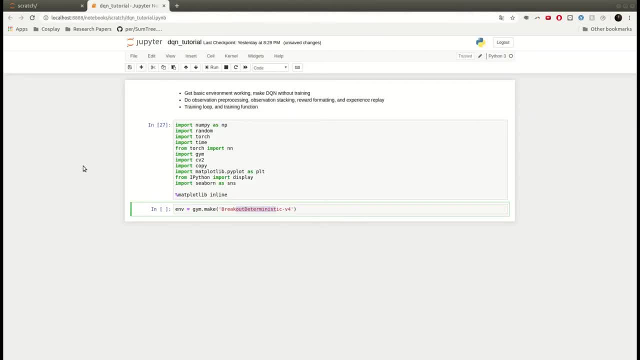 up here. it's like a one player pong, guess. i kind kind of uh cool. so first we want to figure out what are the actual state and action spaces of this right. so a state space is what are all the possible states we can be in. in other words, in our case it would be what are all the possible. 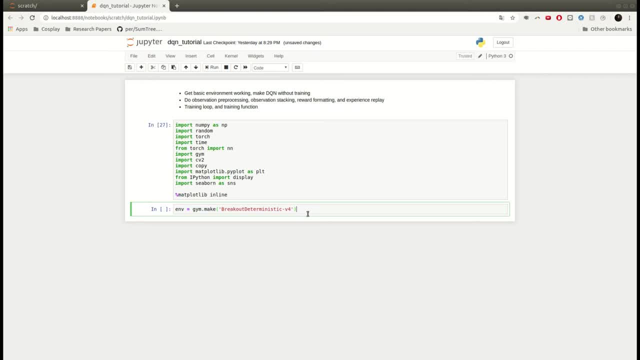 arrangements of pixels. and then the action space would be: how many actions do we have and what are they? so in our case, i think we have four. it's a no operation, a start game, go left and go right. i think we can. we can confirm this with actually this right here, right, so we can print this out. you just do an maction. 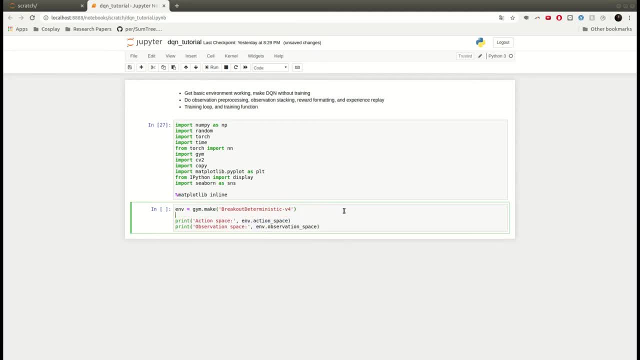 space and an mobservation space, and now, when we run this, we should make the environment and also get these. so this was correct for discrete actions. and then a 210 by 160 image with three channels. so that's for your rg and b values. so this will be the shape of our images. now we can actually get. 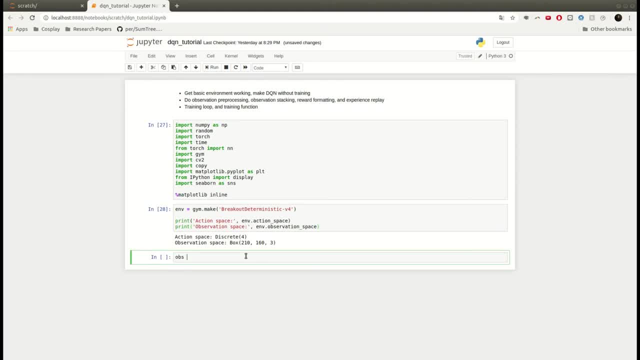 our first observation, an observation right, it's just like a state. so we say, obviously, observation equals mreset, And if we do this, we can actually print this right now. So this is what this has done. It started a new rollout or a new episode. Episode basically just means like a. 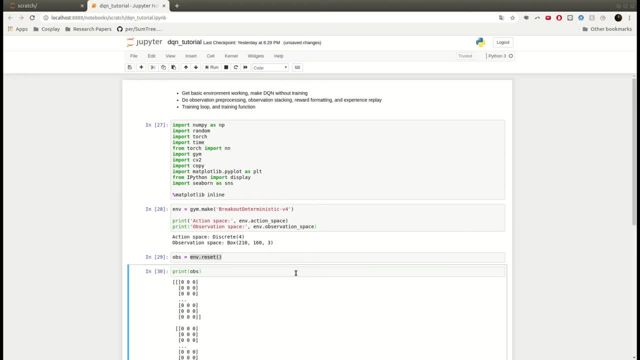 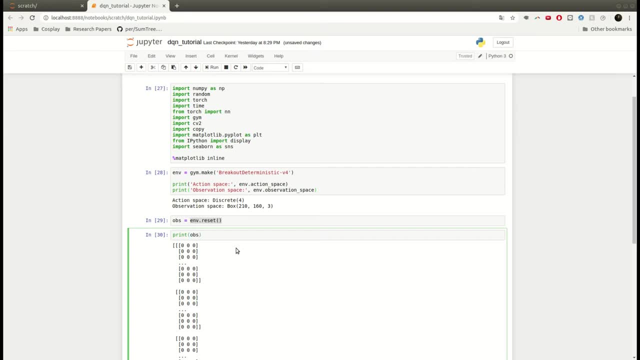 playthrough of the game. right, So we print out observation right now. We should get a bunch of pixel data. It's mostly zeros because the majority of the screen, I believe, is black, or about half of it. We can print out the shape. We should get the same thing as we got right here, right, Cool? 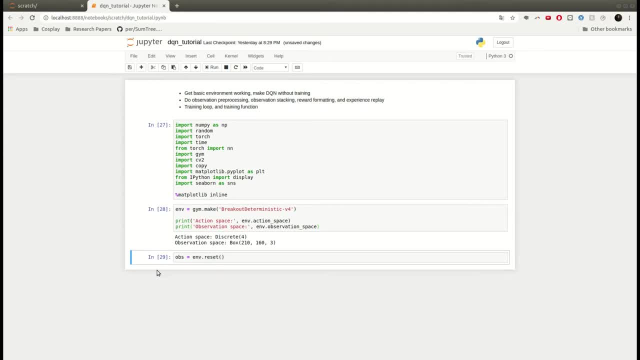 So that's all good, Just sanity check right there. And now what we actually want to do is we want to essentially be able to play out episodes of this game, or essentially, we want to be able to play out rounds of the game. So then we can get data and we can use that to train our model. 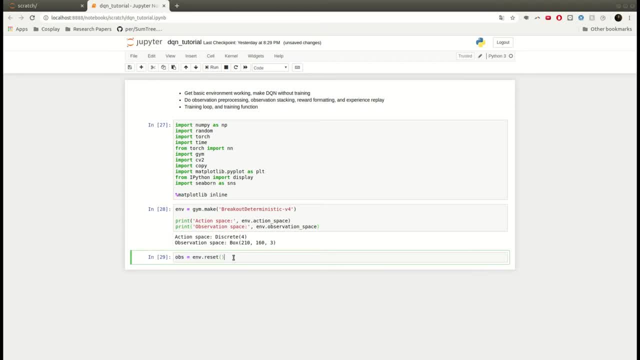 that we will create. So the way we do that is: first, we should probably define a max number of steps. We do this so that maybe the environment- or sorry, not the environment- For example, if we were to have a policy that kept choosing just no op and did nothing, the 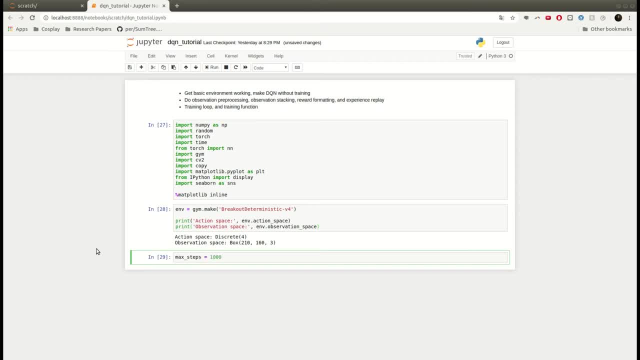 entire time. we would have a policy that kept choosing just no op and did nothing the entire time. So if we were to have a policy that kept choosing just no op and did nothing the entire time, the game might never end. So just to have a limit there And then essentially what we want. 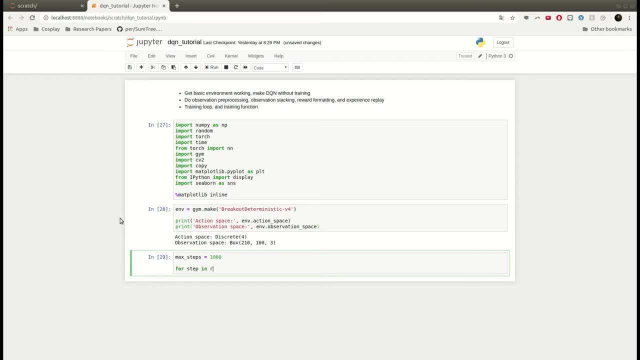 to do is loop through and say four step in the range of max steps. The first thing we want to do is to choose what action we want to take, right? So that's going to be one of four actions. Right now we're just going to choose randomly. Eventually, our agent will be choosing this. 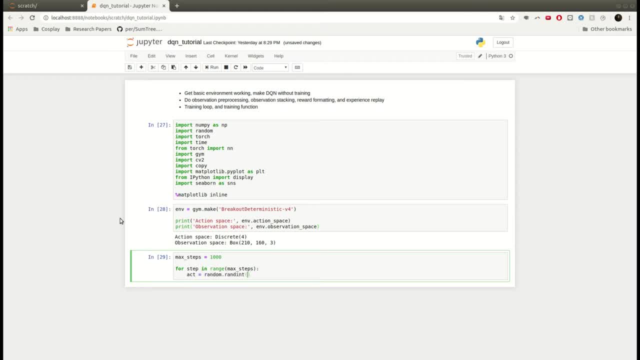 for us, right. But for now we are just going to get a random integer between zero and three and inclusive. So zero would be the first action, Third would be, three would be the last. Now, once we have our action, we can enact that in the environment. So to actually enact our action, 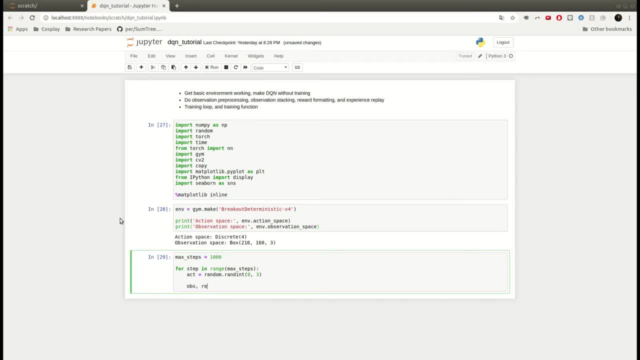 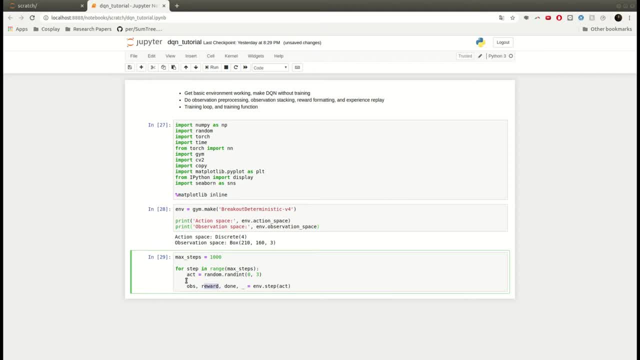 And then done. we'll essentially tell us whether or not we have reached the last sort of state, whether or not this was the last state, if the game's over or not, And then we don't care about this part right here. I think it's just extra info, Cool. So what we can actually do is we can. 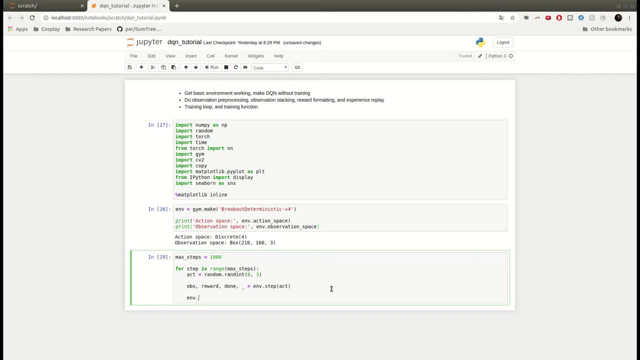 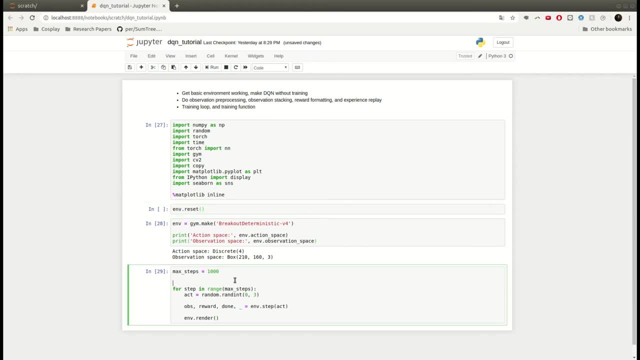 see this playing out now. right, So we can test to make sure this works by saying: mrender, This will actually show us the environment. We can actually test that up here, right, If we say: mreset, Oh yeah, we will want to do that here, mreset, right, Because this restarts the match. 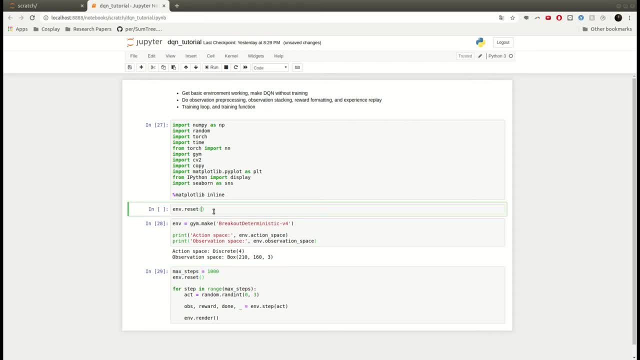 basically, and puts us in a fresh state So we can do mreset, and then, mrender, And if we just run this right here, we should get, yeah, just sort of this. Oh, just appeared on me, Oh, actually. 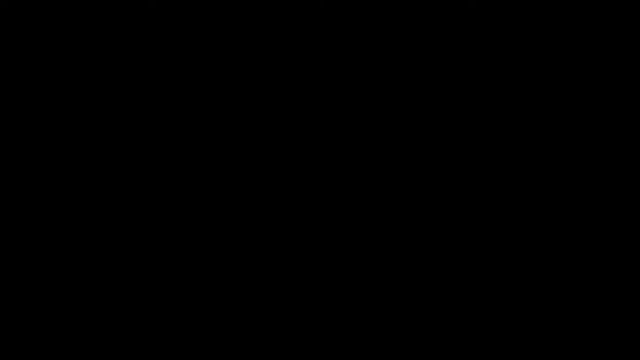 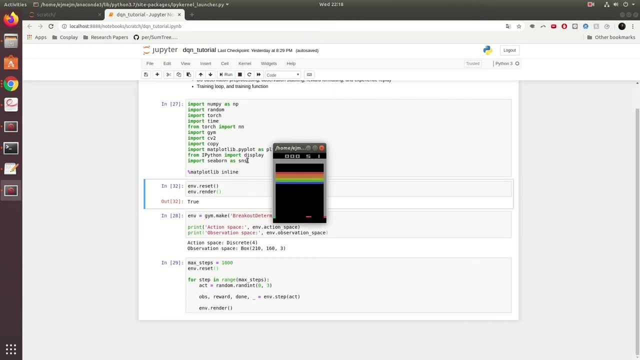 one second. I may need to fix this So you guys can see it. Okay, I am back. I just need to make sure that this was appearing. So this is what happens when we render this, So I just had to adjust my settings there. Now that 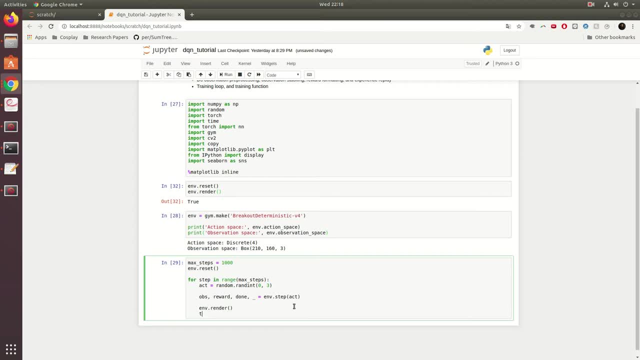 we have that, we can move on and we can actually say we want to add a little delay in between these. So let's add a 0.05 second delay. I'm going to add a delay between rendering for each loop, or else it's just going to go way too fast for us to understand what's happening, And then we'll 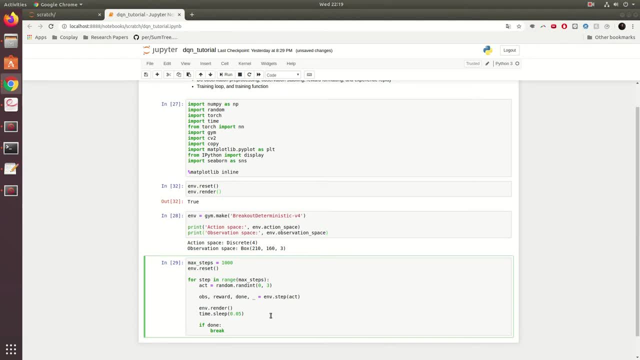 go ahead and finish this before. Essentially, if we finish the episode before we hit the max- yeah, before we hit the max number of steps, we do want to stop running this. So now, if we run this, we should see our agent playing There. we go Already missed that. Oh, nice, nice It's doing about as. 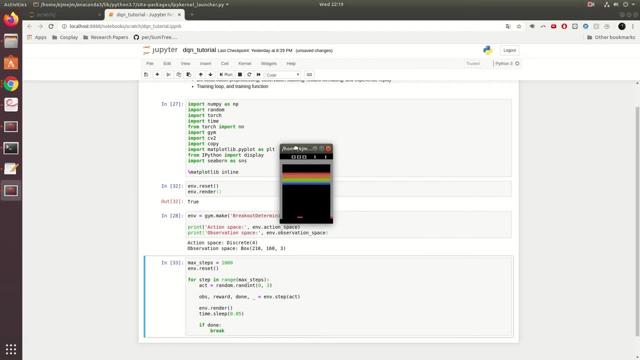 well, as you would expect for having random actions, but it works. So there we have our environment working, And the next thing we want to do is we're just going to quickly set up our QNet work architecture. I'll be using the same parameters as in the original 2013 paper. 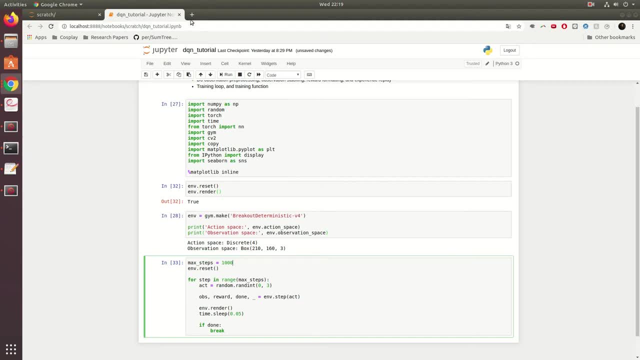 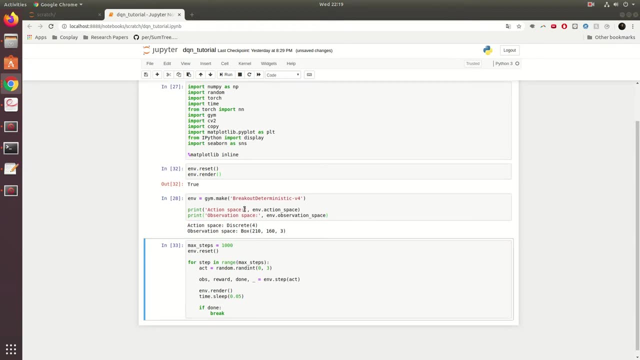 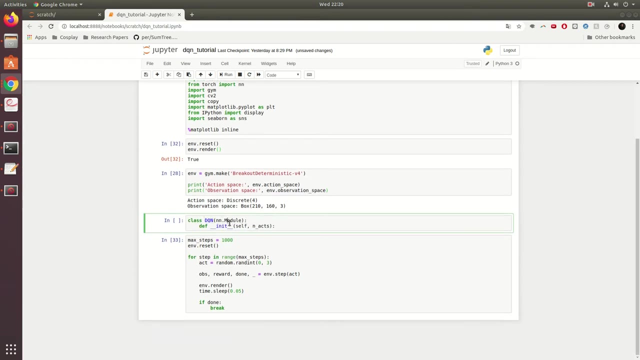 which I will link in the description, as long as I remember. So let's actually make that. So we are going to do that right here. So we're going to create a new class, call it DQN for deep Q network, And, right, we're going to be trying to predict Q values for this. And if you 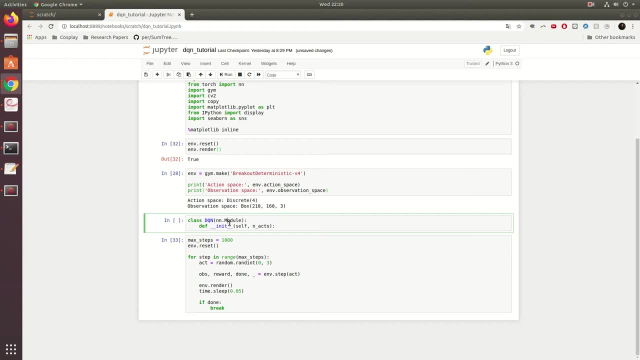 remember, Q values are essentially our expected reward over the course of our work. So we're going to be trying to predict Q values over the course of a whole episode, right? So we play out our game and the we're trying to predict from a given state how much. so not, not from the whole. 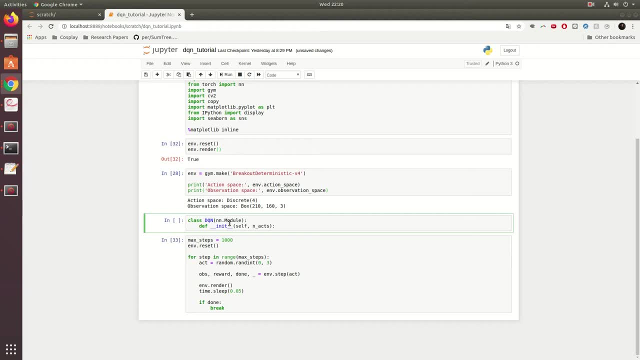 episode, but from the current state, right. So we'll be trying to predict, given a current action we take in a current state, how much reward do we expect that to generate? right, Because if we can predict that, all we have to do is take the best actions right, The actions with the highest. 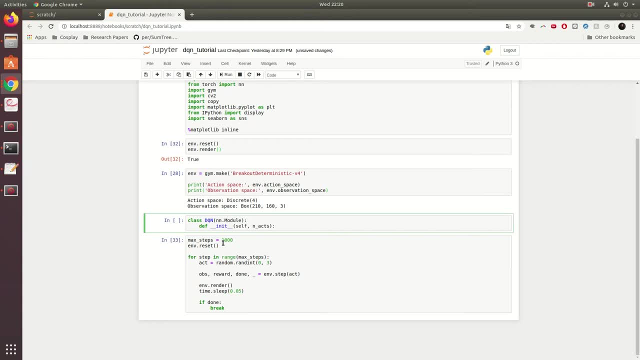 Q values, ideally, um, to get the best results. So we are going to be predicting the Q values over the course of the course of this and I imagine this is going to be a little bit harder and it's going to be a little bit competitive, but we've done it. So again, remember, we can't keep. 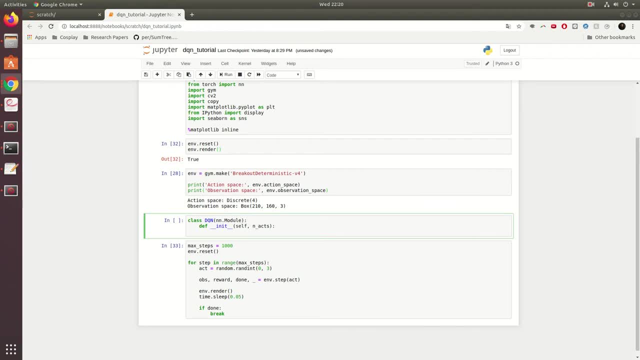 all these in a table. We have so many possible states, because we're now working with pixels. right, It's a, it's a continuous environment, Um, so we have to use prediction, Uh, so let's make this. So we're just going to basically make a convolutional architecture. Uh, if you don't know, 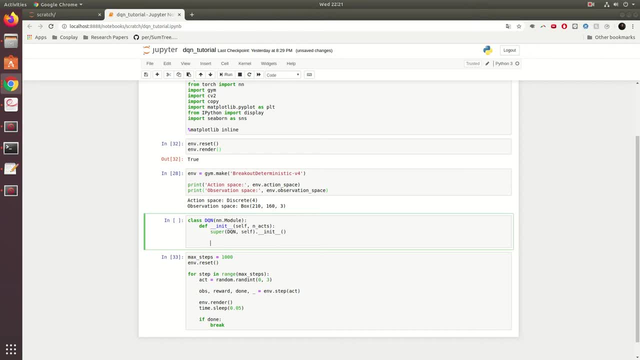 what a convolutional neural network is. I recommend you look that up, or you can just assume it's a black box where you give it an input and an output. Um, you know that works too. Uh, I won't be. so these are the layers we're going to use, right? so we're going to have three convolutional layers. 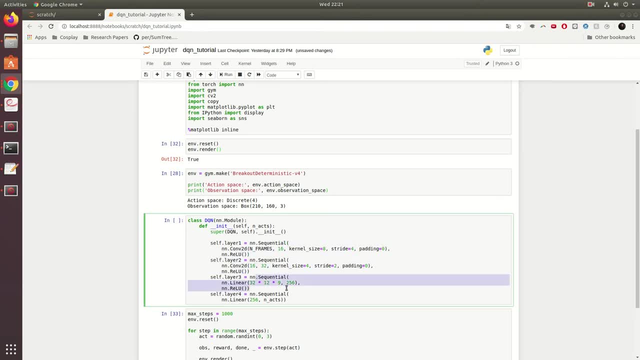 or no, two convolutional layers and one linear layer. um, so we have, we start out with. so i define in frames here. i don't think i've defined that yet. um, what we're going to end up doing is we're going to end up stacking frames, for right now, we'll just leave this as one and we'll actually 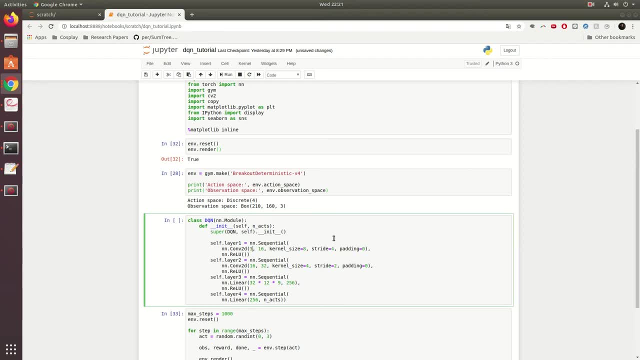 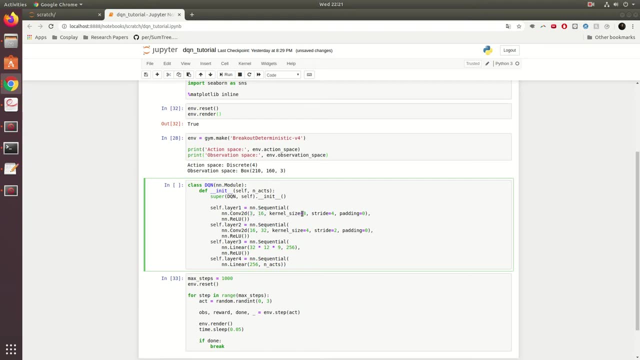 we'll leave this as three because we have three rgb channels. we'll come back to this later and fix that up, but, um, what we have now is we have: we're going from our rgb layer to 16 filters with a kernel size of 18- a straight of four. um. then we go up to 32 filters- a kernel size of four straight. 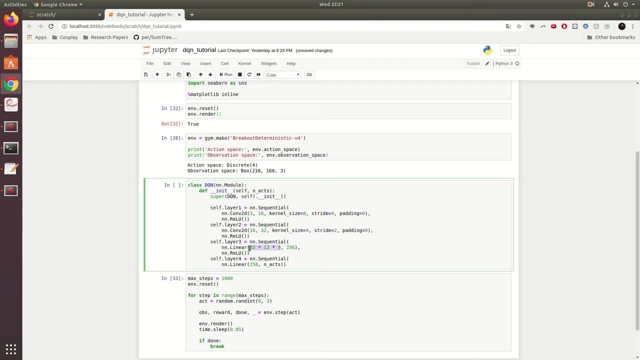 of two. and then we have a linear layer that is: oh, this might actually be incorrect. no, this is correct, this should be correct. um, uh, we're going from this many units to 256 units. we are, by the way, using relu activations for all of these. and then our final layer. 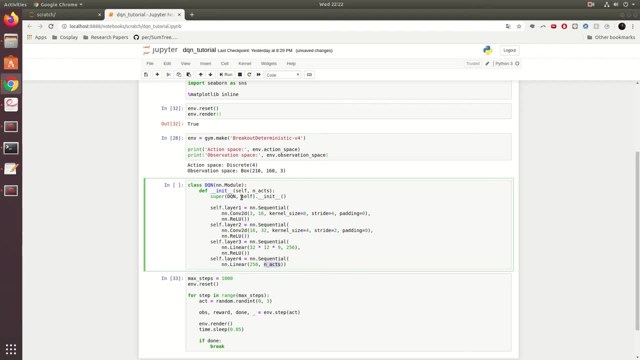 we just do a linear to the number of actions we have and the inactions we are going to take in as a parameter. so the very standard um thing here. the next thing you want to do is just define the forward pass of this and again, if this is confusing to you, definitely go back and watch. 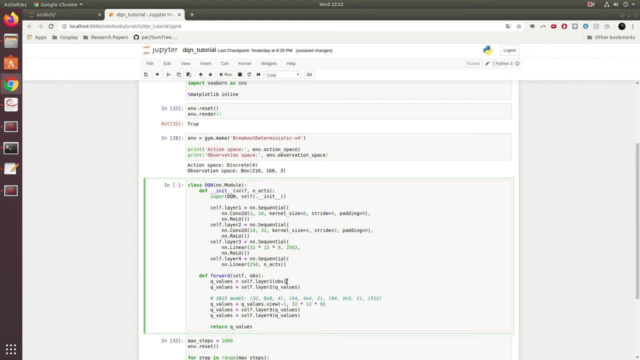 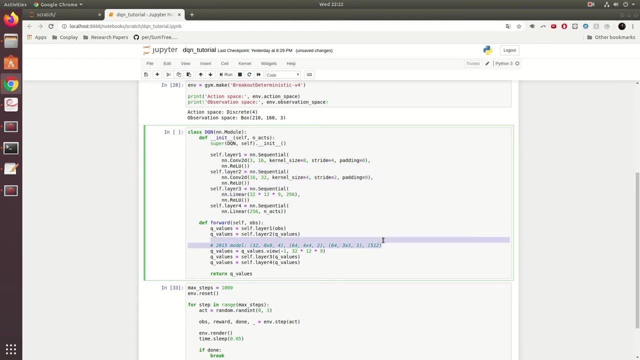 my tutorial series on just creating neural networks. i don't explain convolutional neural networks, but i do explain sort of just fully connected neural networks, which will help, and then you'll probably want to look up convolutional neural networks, but anyway, i don't need that. so what we want to do is we have our four layers, we just want to pass in. 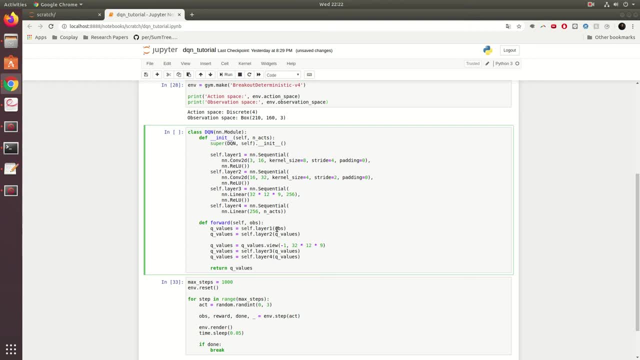 once we get an observation, we want to pass that through um, our first layer, our second layer. we'll then reformat this to flatten out our data. right, because we were just passing it through convolutional layers. we need to flatten it out so we can now pass it through our third layer, which. 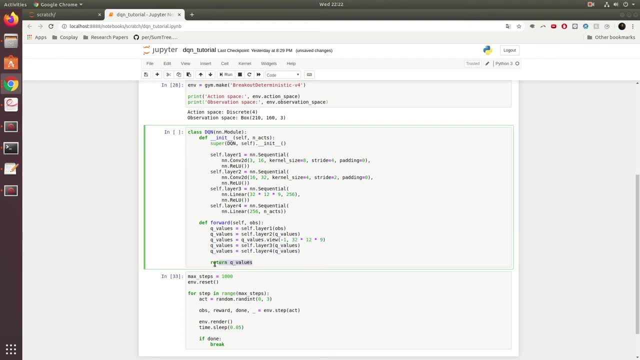 is a fully connected layer. then our fourth layer, then id. ideally we should get our q values, so we should be able to run any sample. let's just make sure that we're doing it right. so we're going to make sure this works right. so let's create a new dqn goes dqn in our case. we have four actions right. 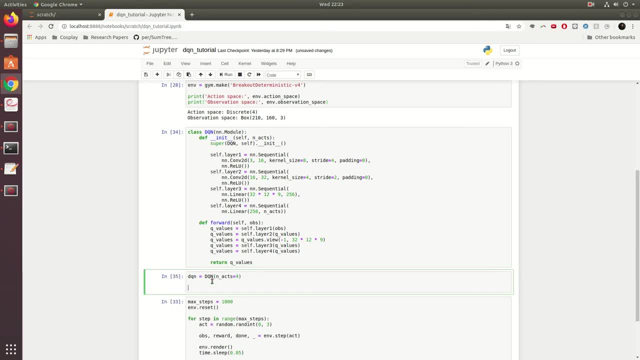 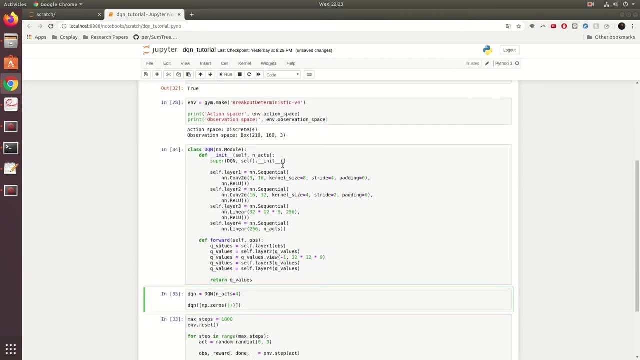 let's make sure that runs looks good. now we can ideally actually pass through a, let's say, np.0s, and what is the shape of this going to be? it's going to be- what was it again i'm forgetting? um, we are going to be actually resizing this. that's something i'm 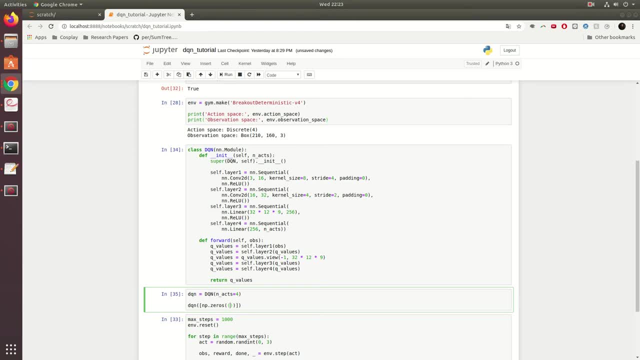 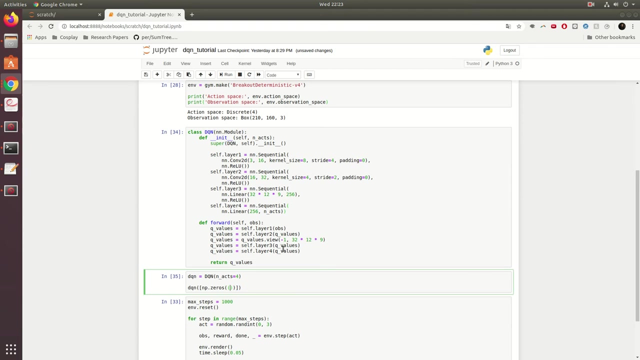 going to be doing. i think i forgot to mention um. we will be resizing our images, so we start out with 210 by 160.. um, let me double check what i did in my reference code. i believe i did 84 by 110, or is it 110 by 84? oh gosh, we'll just try both. um. it's got to be one or the other um in the regional. 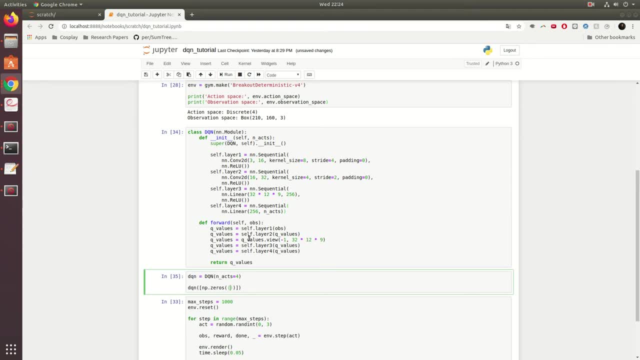 paper they actually use 84 by 84. they size it down to 110 by 84 and they're going to be able to then crop it down. uh, we won't be doing the cropping. the actual reason they cropped it was just because of the fact that they- it was just a limitation of libraries at the time. we don't. 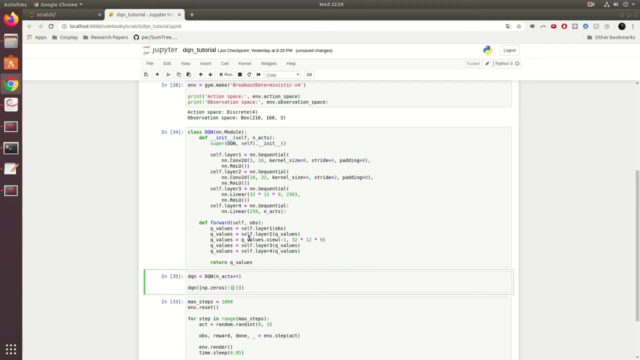 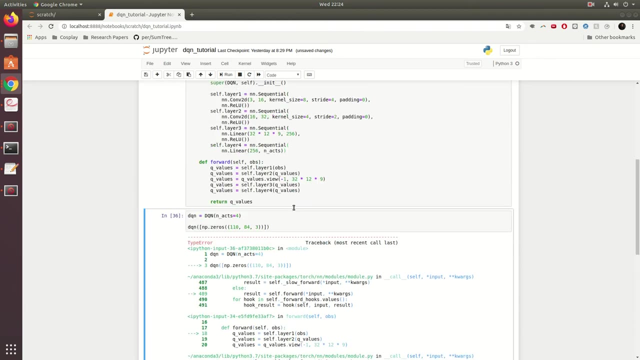 have that limitation anyway. i'll go more into detail on that in the next episode, but i believe this should be 110, 84, and then we have three channels. so this is just what, the same shape as what our input will be right, let's make sure this works. it does not. oh no, i put tensor. oh yes. 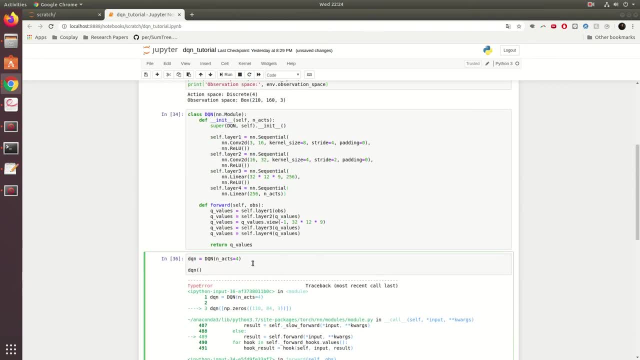 because we need to. this does need to be a tensor. um, actually we should just do: uh, we should put a one in front of this, because we're passing one example through. so we'll say in: oh, that doesn't work. um, oh, uh, input data will equal. 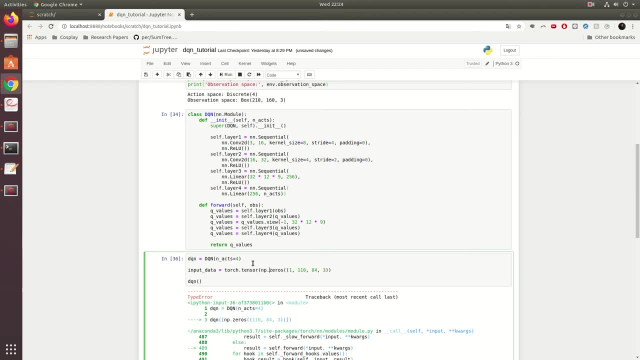 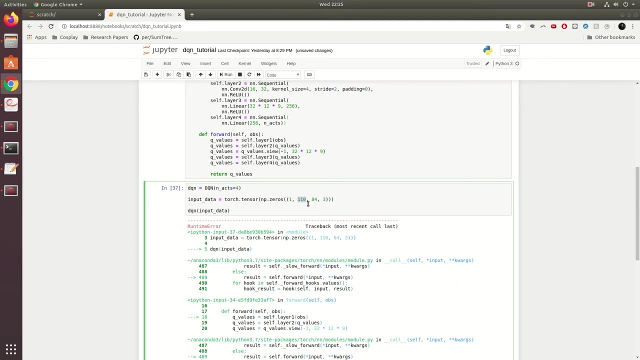 twitchtensor. okay, i don't think we actually need the np.0s here, but i don't care. um one more time, what's our issue now? ah, it must be 84 by. oh, that's right. so i i knew to pie torch, i forgot you're supposed to put the channels first, right? so we have three channels: 84, 110, is it? 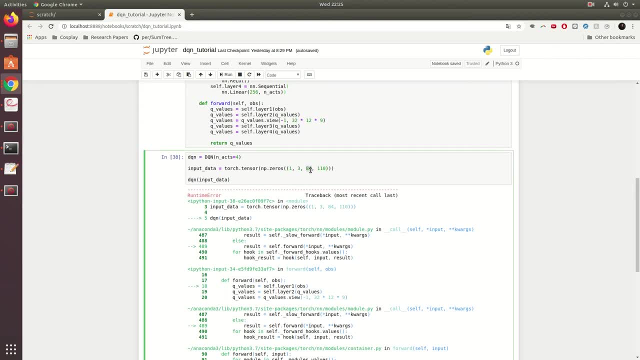 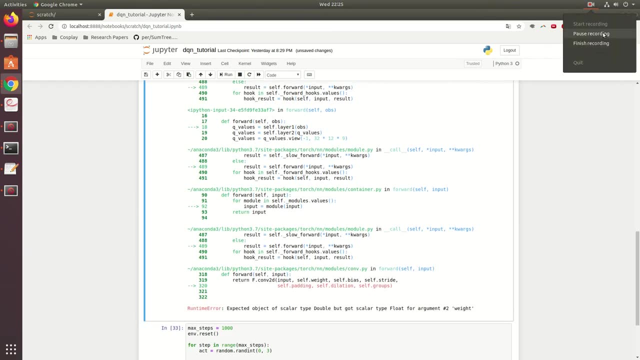 oh boy, what's happening? 110 by 84? i don't think that was there, but okay, i'll be right back as soon as i figure out what's going wrong. okay, i am back less than a minute later. all we need to do is add a dot flow right here. 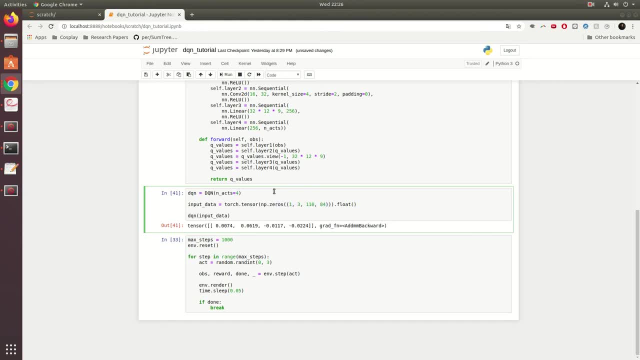 to our um. i guess this was interpreted as a double, whereas the qnet, or our network, was expecting floats or something along those lines. so now, if we pass it through, as you can see, we do get. we do get a tensor with four values. awesome. so these are our estimated q values. as you might have noticed, they 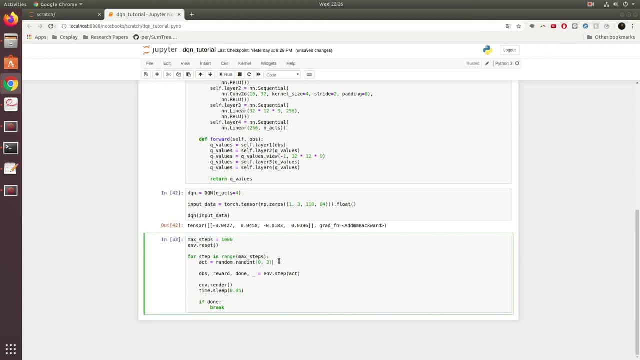 are completely random right now, but in the future, what we want to be able to do right is: we want to come here and we want to say, first we want to create our dq, and then we want to say, basically, dqn, or like our action will equal our dqn, and then this will be our observation, or we: 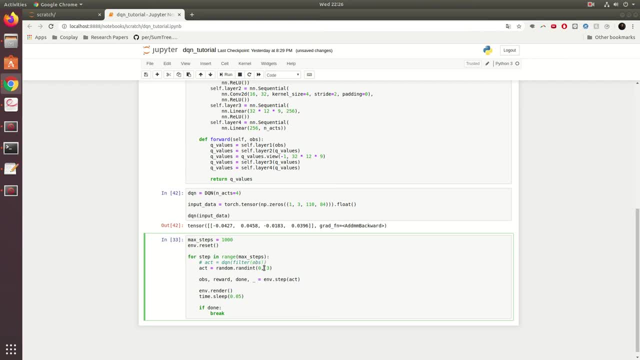 should say: we'll have some filter function right and we'll pass. our observation is that that will go into our dqn and we'll get not an act, we'll get a q values and then our act will be something like: act equals the arg max. i think you can do it into the arg max, right? um, i'm actually not sure if 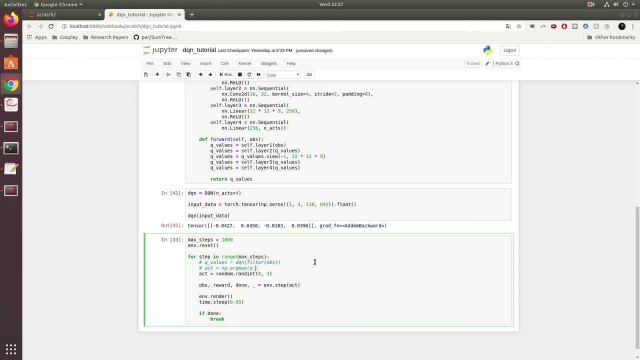 you can do arg max. i'm going to assume you can. we'll get back to that, though i'm going to assume, uh, of the q values, each steps here there. um, yeah, so it'd be something like this: right, so we get our q values and then we take the max. 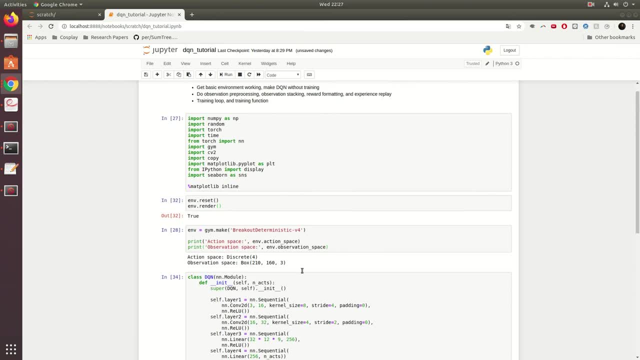 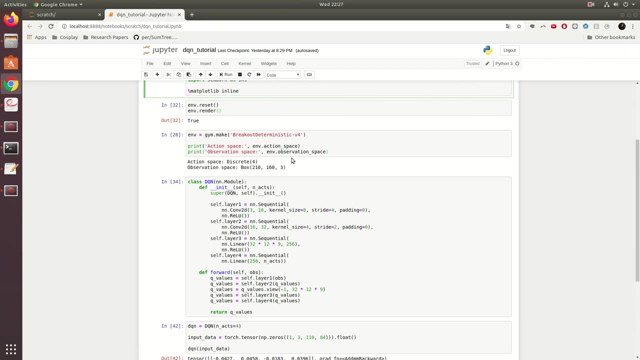 and then that's what action we take. um, so this is essentially what we're building up for. i am going to cut us off here because, even though i don't think we've gotten through too much yet, it's, i think it's still a lot to take in. there's going to be a lot more. the next episode is also. 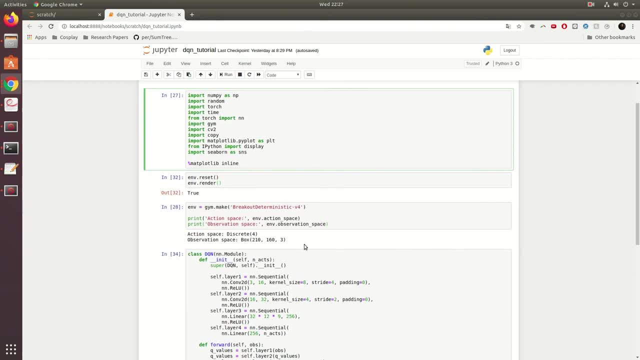 going to sort of fall into the next episode. so we're going to sort of do that, but i'm going to ramp up this a little bit, so let's just go through a quick summary before we end this up. first, of course, just importing libraries. then what we do. we don't need this anymore. we create. 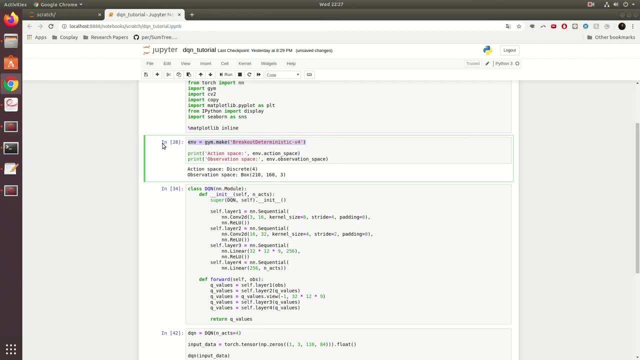 our environment, which is in this case an atari breakout environment. we check what the action in observation spaces are. we see that we have four possible discrete actions, so zero through three are our action choices, and an observation space of 210 by 160 by three, which essentially means we 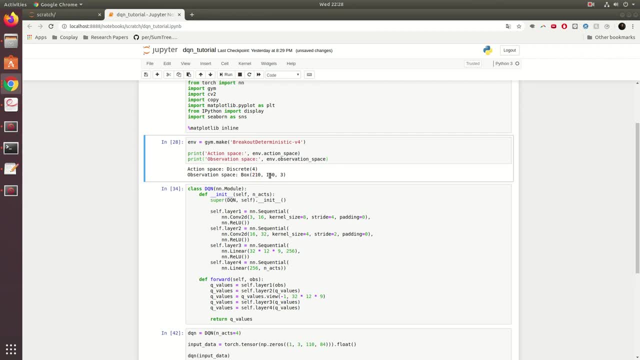 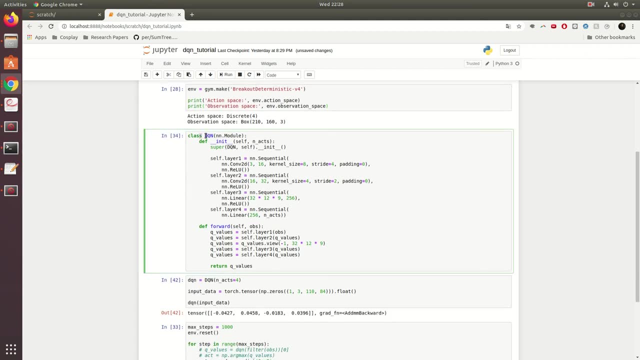 have a pixel, we have pixels of this width and we have pixels of this width and we have pixels of this width, this height, or is it backwards, i don't know um, and then our rgb channel. what we did then is we created a archit, our architecture for our deep queue network, which will essentially be: 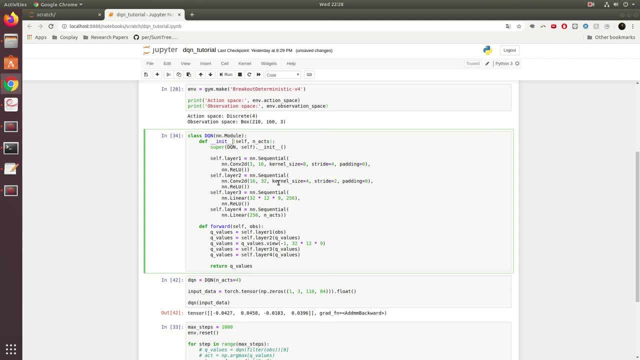 predicting q value. q values- oh, i can't say it right now- and this takes in our pixels. that said, that means that we will resize this to a smaller size. we pass that through through this forward function and we get out these estimated q values. of course, i think you've all noticed, there's no 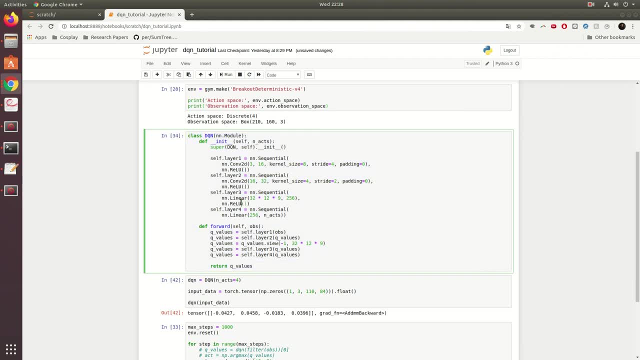 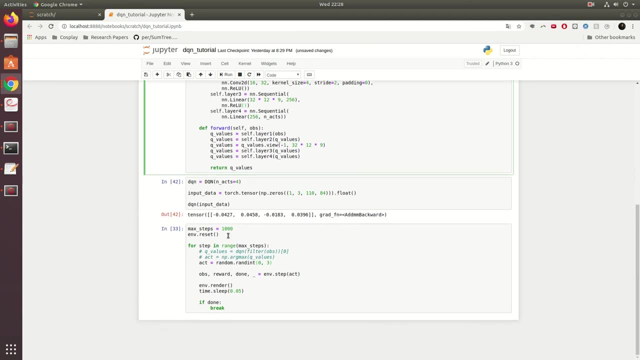 training function here, yet, so this is just going to spit out absolute nonsense, because we will be covering the training in, i believe, two episodes. so what we do then, though, is we go and we create, we reset our environment, essentially starting a new episode or a new playthrough of a game, and then we 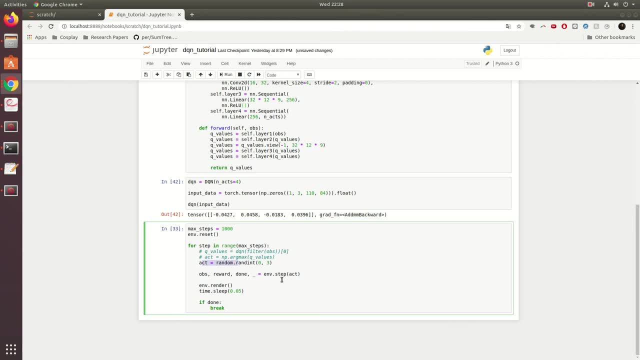 loop through and we choose a random action, enact that action in the environment, receive our new data, including an observation, a reward and a something that tells us if it's. if this is a terminal state, we render it so we can see what's going on. uh, and at some point we end up stopping and finishing the playthrough, so that's all we're.